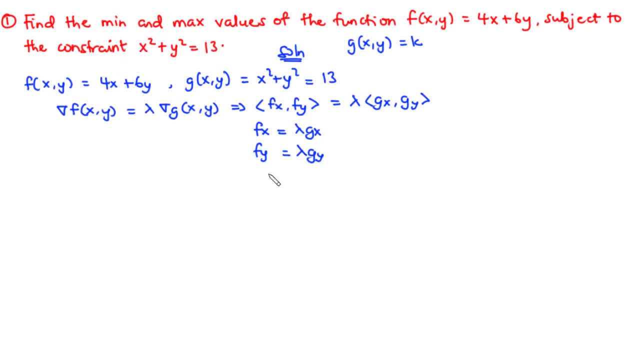 we are going to have our third equation, that is, the constraints. so we have: x squared plus y squared equals 13. So we call this equation 1, equation 2, and then equation 3, and then we have lambda and that is called the Lagrange multiplier. 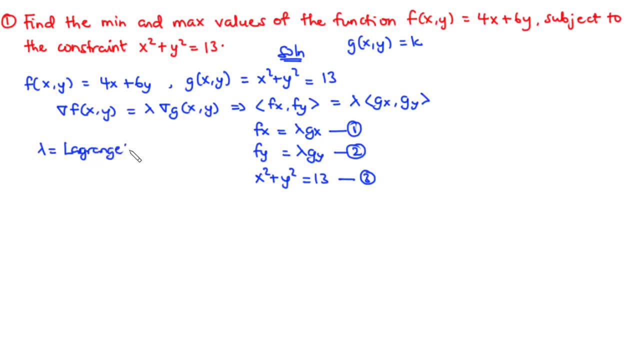 Now from this we can solve this example. So let's try to find fx, fy and then gx, gy. So for fx, that is the partial derivative of the function f with respect to x. This is going to give us 4, And then we have fy, also to be equal to the partial derivative of this function f. 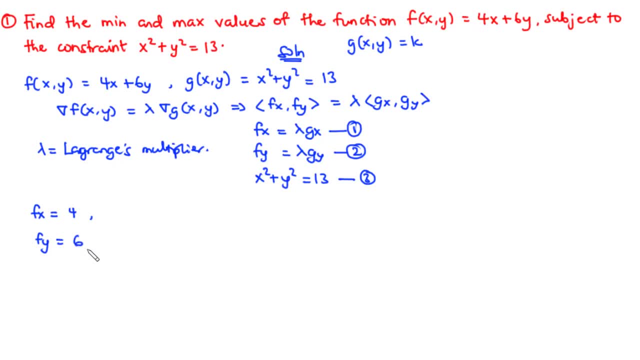 With respect to y, And that is going to give us 6. Also, for gx, we are going to have 2x, And then for gy, we are also going to have 2y. Therefore, we can have fx, which is equal to 4. 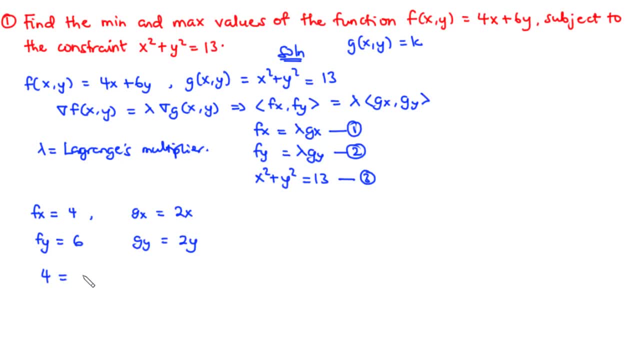 So 4 equals lambda times gx. So we have 2x lambda equation 1, And then we have 6 equals 2y, And then we have 6 equals 2y, And then we have 6 equals 2y Lambda equation 2. 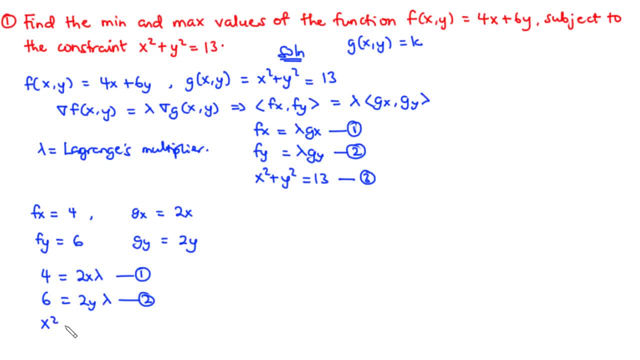 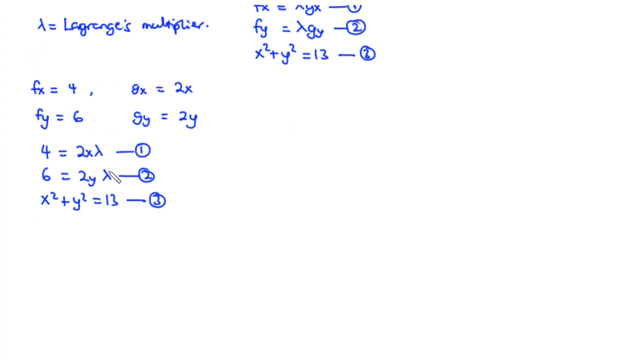 And then we have the constraints. That is, x squared plus y squared equals 30. We call this equation 3. Now, at this point, what we are going to do is We want to find the values of x and y. So, first of all, let's try to make lambda the subject from equation 1 and equation 2. 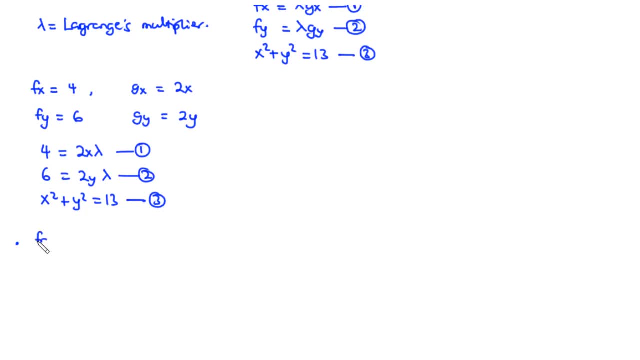 So that is from equation 1. From equation 1 We have 4 equals 2x times lambda. We divide through by 2x And then we are going to have lambda to be equal to 2 over x, Again from equation 2. So from equation 2. 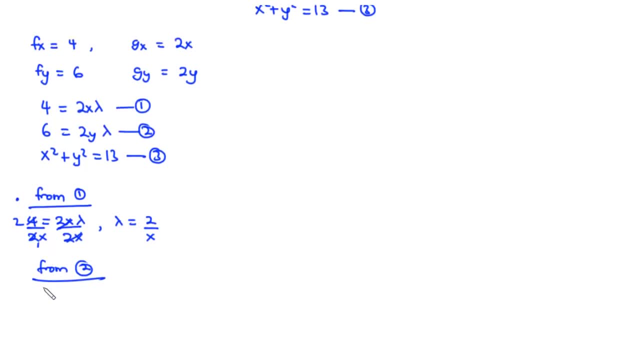 We can also have 6 equals 2y times lambda, And then we have 4 equals 2x times lambda, And then we are going to have lambda to be equal to 3 over y. So we have 3 over y. That is also lambda. 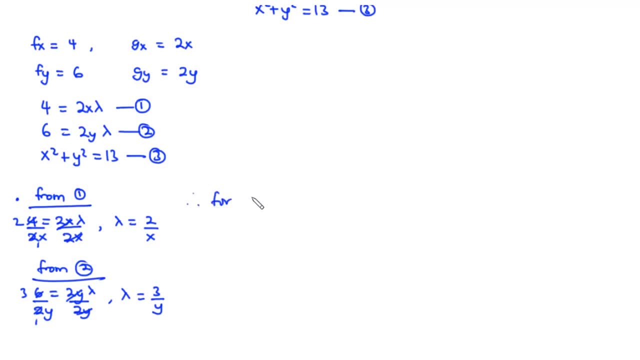 Therefore, for lambda equals lambda, We have 2 over x equals 3 over y. Now here we can choose to make any of the variables the subject. So, assuming that we want to make x the subject, We can choose to make any of the variables the subject. 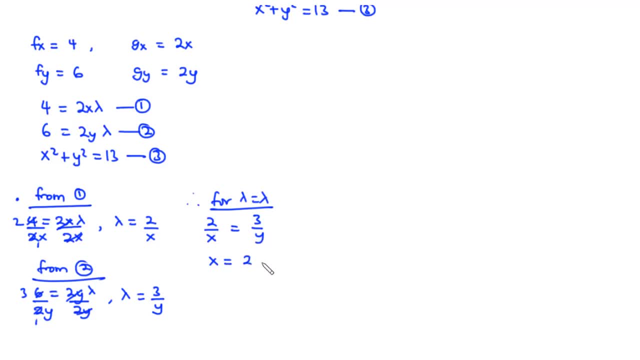 We are going to have x equals 2y, So we multiply 2 by y And then divide by 3, So this is an expression for x. Now the next thing is We are going to put x equals 2y over 3 into equation 3. 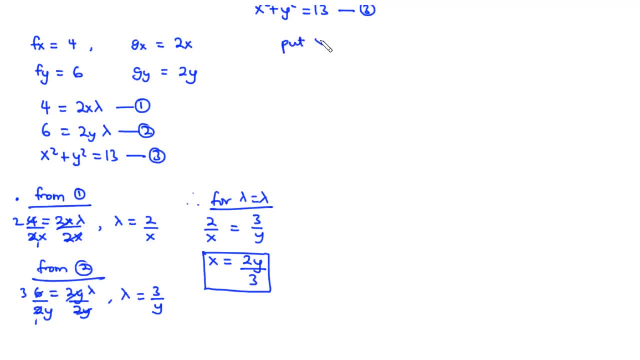 So we are going to put x equals 2y over 3 into equation 3. So we are going to put x equals 2y over 3 into equation 3. So we are going to have x squared so 2y over 3, all squared plus y squared equals 13.. 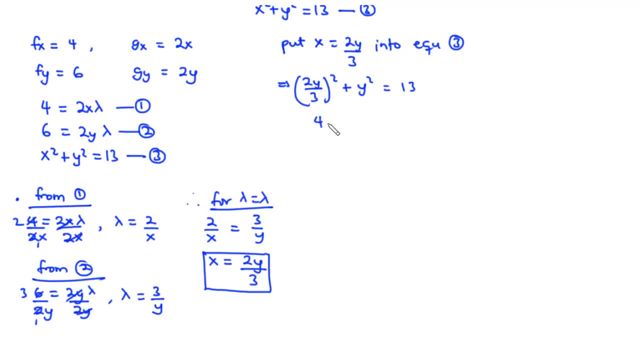 So this becomes the numerator we have 4y squared over 9, and then plus y squared equals 13.. So we find the LCM between 9 and then 1, and that is 9.. 9 divided by 9 is 1,. 1 times 4y squared is 4y squared. plus 9 divided by 1 is 9,. 9 times y squared is 9y squared, and then equals 13.. 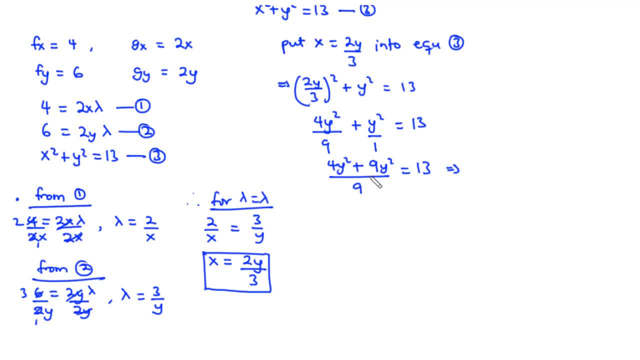 So at this point we cross multiply, and then we have 4 plus 9 is 13,. so 13y squared equals 13.. Times 9,, so we divide through by 13, and then we have y squared. y squared equals 9.. 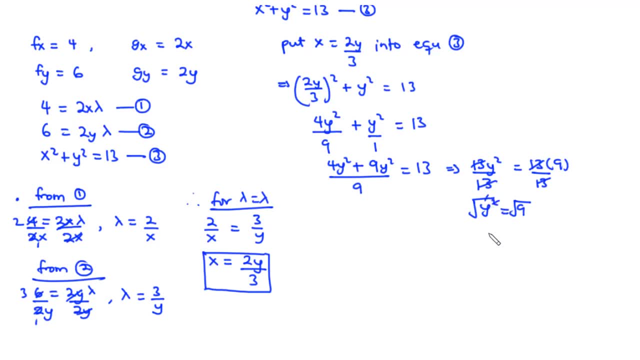 We take the square root of both sides and then we are going to have y to be equal to plus or minus 3. So y is equal to 3, or y is equal to negative 3.. Now for y equals 3.. 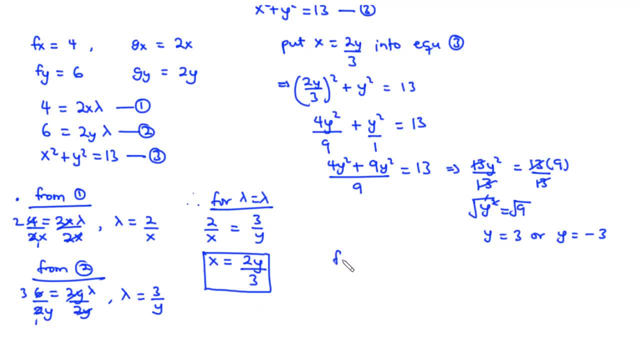 For y equals negative 3,, we need to find the value of x. Therefore, for y equals 3,, we have x to be equal to 2 times 3 divided by 3, and that is equal to 2.. So we have x to be 2, for y equals 3, and then for y equals negative 3,, we are going to have x equals 2 times negative 3 divided by 3.. 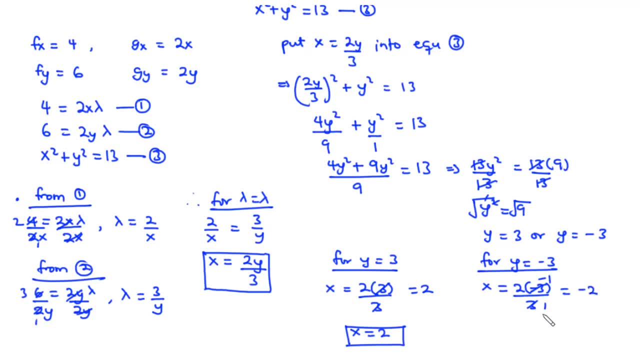 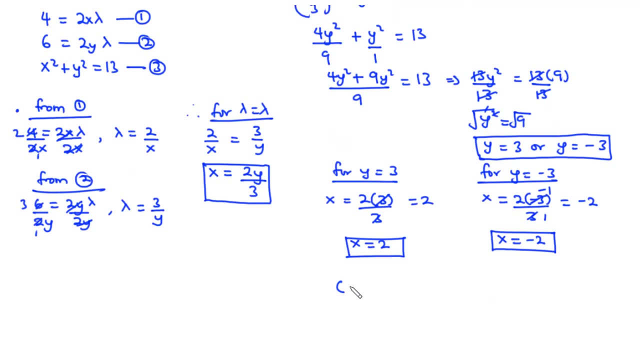 And that is equal to negative 2.. So we also have x to be negative. 2 for y equals negative 3.. Therefore we obtain two points, which are the point 2, 3, and negative 2, negative 3.. 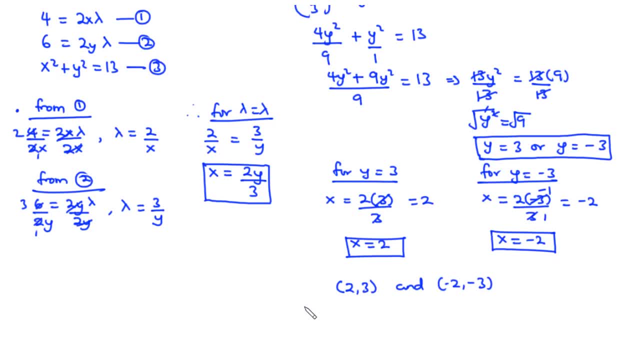 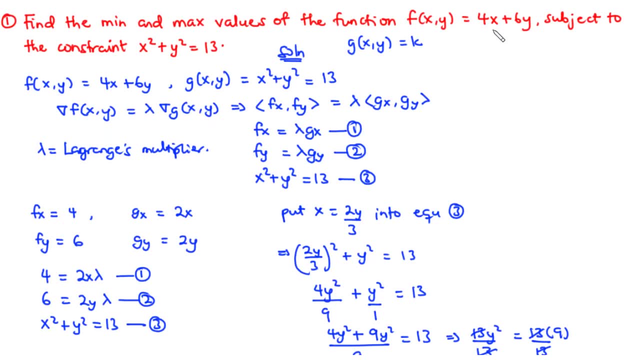 Now we need to find the values of the function at these points. So we have f of 2,, 3. And that is equal to now we have the function f of x, y, to be 4x plus 6y. 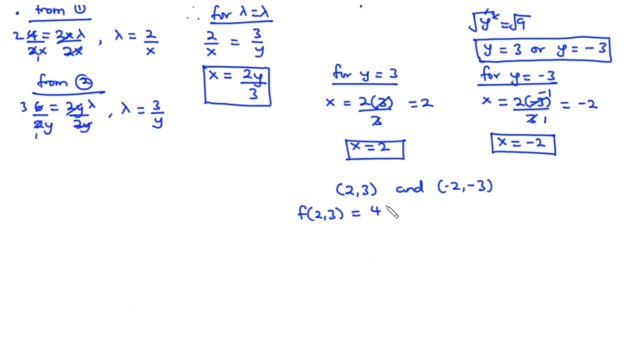 4x plus 6y, So we have 4 times x. in this case we have 2, plus 6 times y. in this case we have 3.. So that is equal to: we have 8 plus 18, and that is equal to 26.. 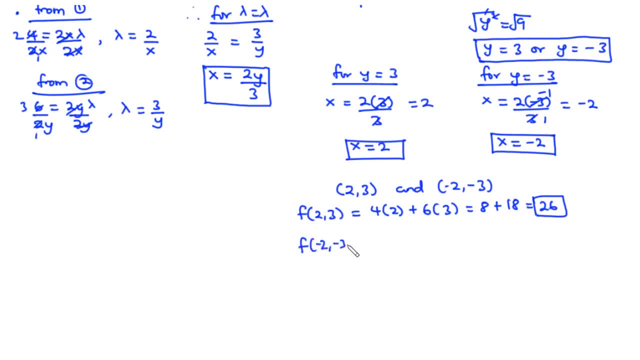 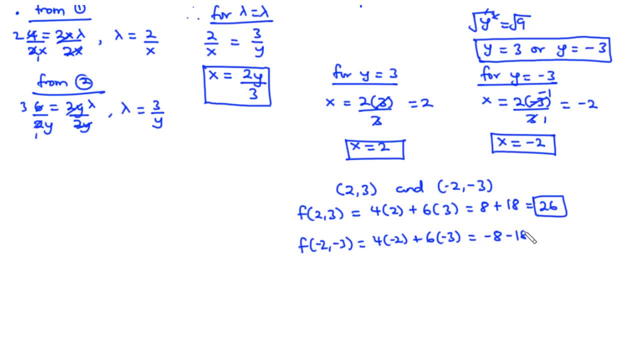 And that will be equal to negative 8 minus 18.. And that is equal to negative 26.. So we have 26 to be the maximum value And then negative 26 to be the minimum value. So the maximum value 26 occurs at the point 2, 3.. 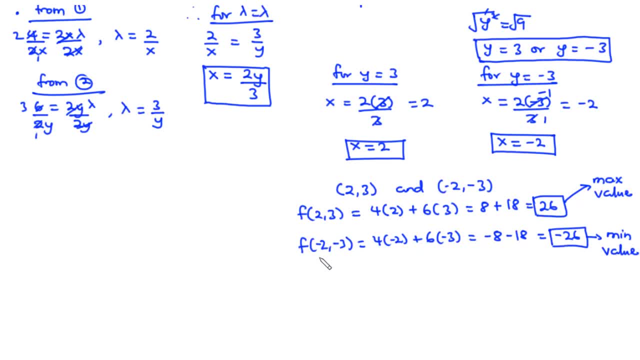 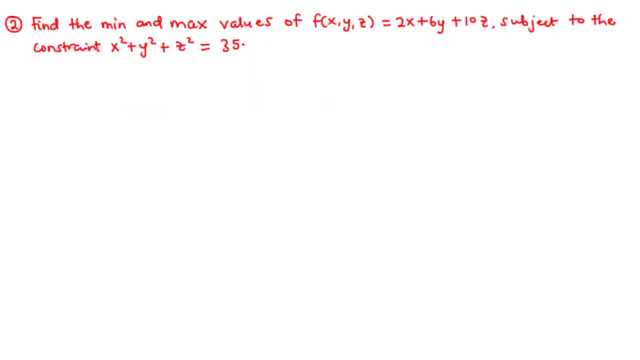 And the minimum value negative 26 occurs at the point 2, 3.. Now let's move on as we solve the second example. For example 2,, we are going to find the minimum and the maximum values of the function f of x, y, z. 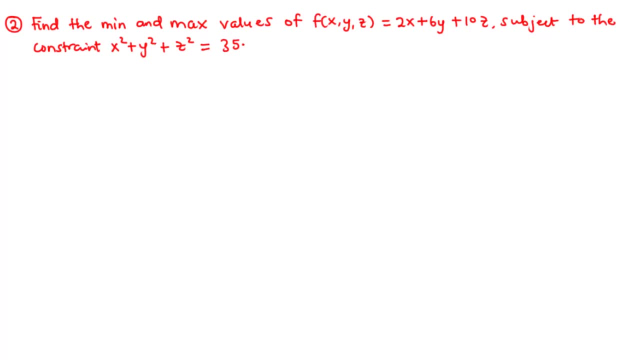 Subject to the constraint, x squared plus y squared plus z squared equals 35.. So here we have a function of 3 variables. Therefore, we are going to have the vector equation to be the gradient of the function f of x, y, z. 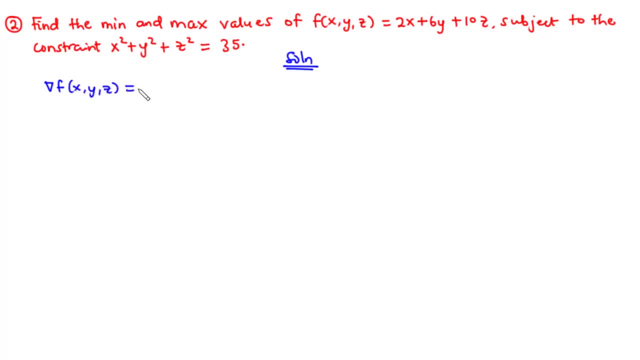 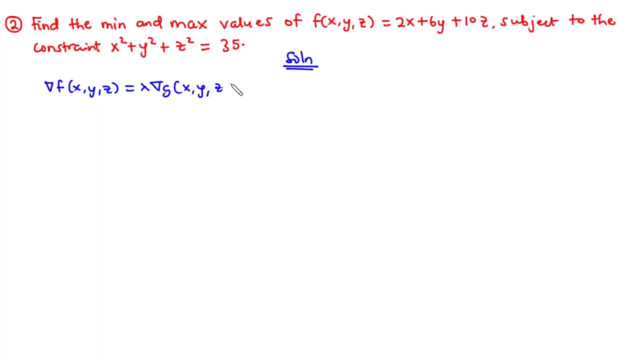 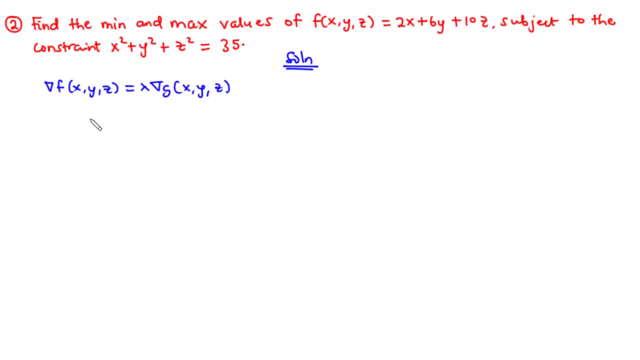 Therefore, we are going to have the vector equation to be the gradient of the function f of x, y, z. Therefore, we are going to have the vector equation to be the gradient of the function f of x, y, z, then gen z. therefore, for fx we are going to have 2, fy we have 6 and then fz we are going to have 10.. 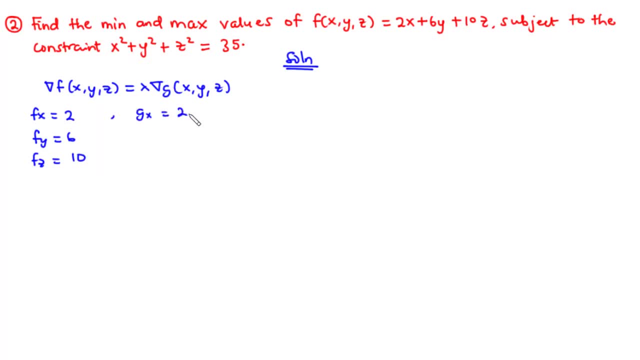 now also, we have g x to be 2x, we have g y to be 2y, and then we have g z also to be 2z. therefore we are going to obtain the vector equations. we have 2 equals, so fx equals lambda times gx, so that's 2 equals 2x lambda, and then 6 equals 2y lambda, and then 10 equals 2z lambda. 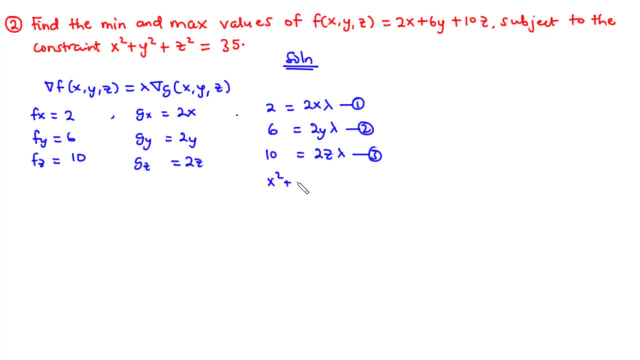 and then we have the constraints: x squared plus y squared plus z squared equals 35. that is equation four. now, like we did in the previous example, we are going to make lambda the subject in the first three equations. so so, from one from one, we have two equals two x lambda. 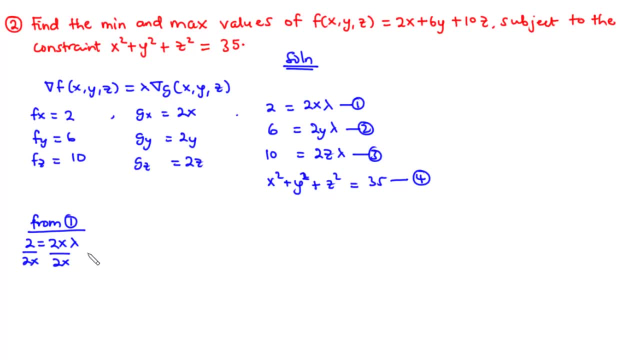 we divide through by two x, and then we have lambda to be equal to one over x, one over x. also from equation two, we have six equals two y times lambda. we divide through by 2y, by 2y, and then we also have lambda to be equal to. 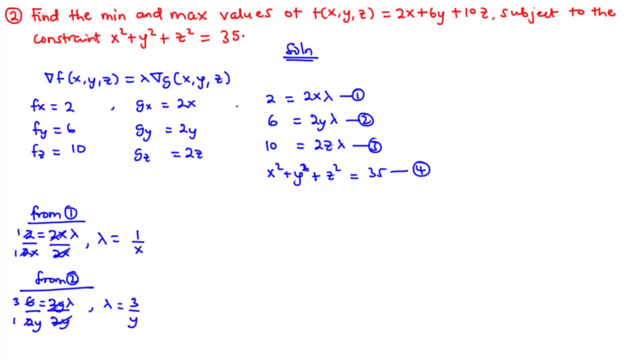 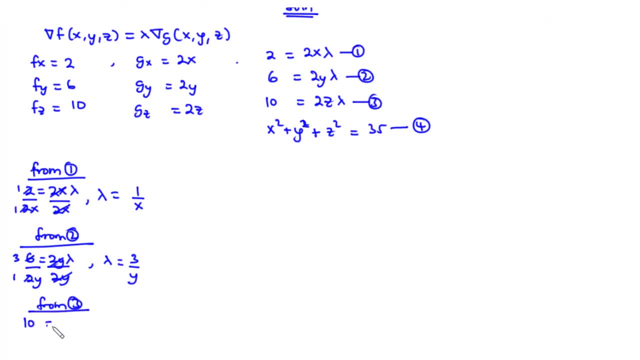 five over x is equal to 3 over over y. and then from equation three we have 10 equals to z. lambda we divide through by 2z and thus we have lambda also to be equal to 5 over z. so now we have lambda to be equal to 1 over x, equals 3 over y, equals 5 over z. 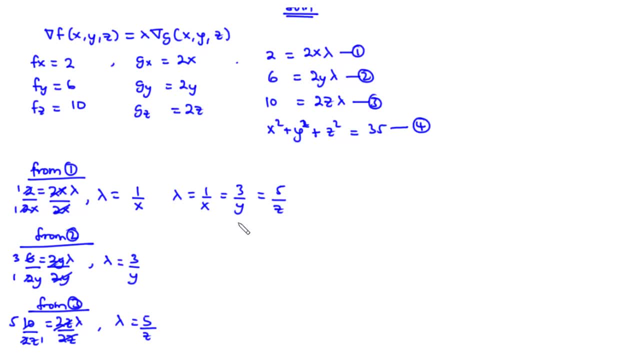 now, from this we are going to create two new equations, that is, we are going to make y and then z the subject in terms of x. so for 1 over x, for 1 over x equals 3 over y. we are going to make y the subject, we are going to have y to be equal to, we multiply x by 3 and then we have 3x divided. 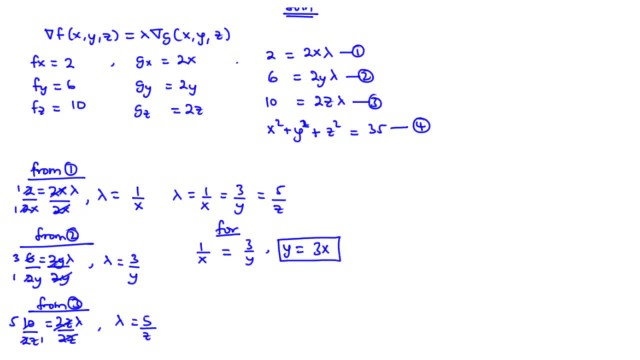 by 1, so that is still 3x. so we have y equals 3x. and also for 1 over x to be equal to 5 over x, 5 over z, we also find, or we also, we also make z the subject, and thus we have 5x over 1, which is: 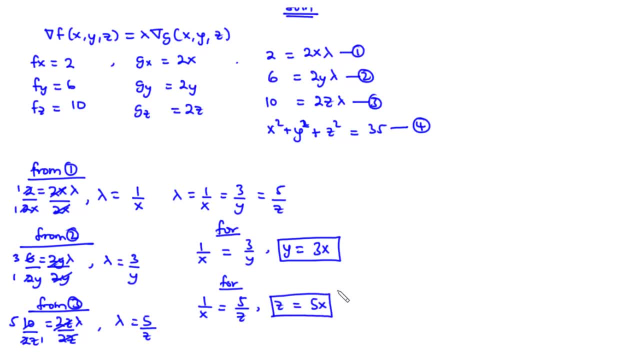 simply 5x. so at this point we are going to substitute y, the expression for y, and then z into equation 4. into equation 4, therefore, we have equation 4. from equation 4 we have x squared plus. into equation 4, in place of y we have 3x. so 3x all squared plus 5x all squared, and that should be equal to 35. 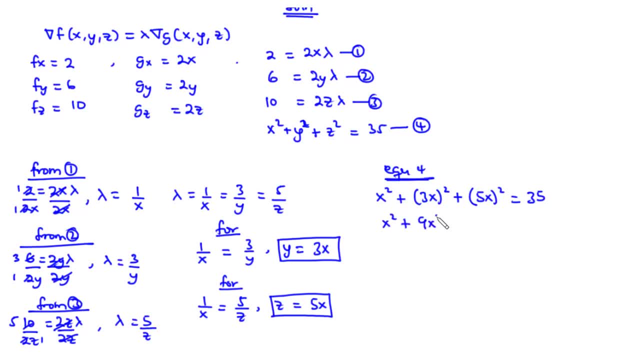 so this becomes x squared plus 9x squared plus 25. x squared equals 35. now, 1 plus 9 is 10, 10 plus 25. we have 35. we divide through by 35 and then we have 1 over 1, which is simply 1. therefore we have x squared equals 1. we take: 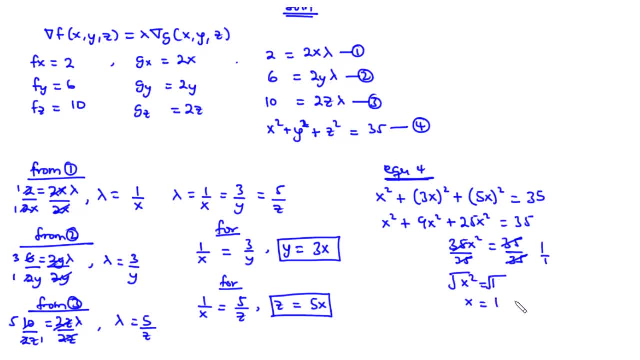 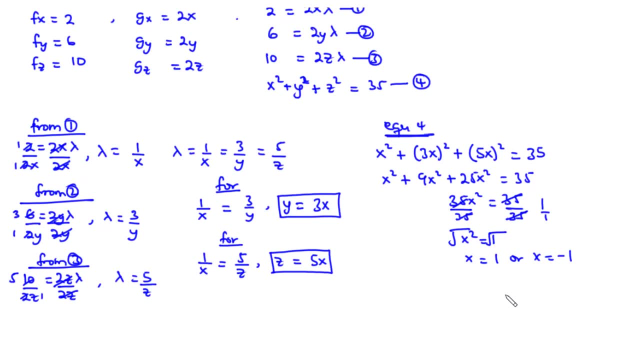 the square root of both sides, and then we have x to be equal to 1 or x equals negative 1. now, for x equals 1, x equals negative 1, we need to find y and then z. so for x equals 1, we are going to have: 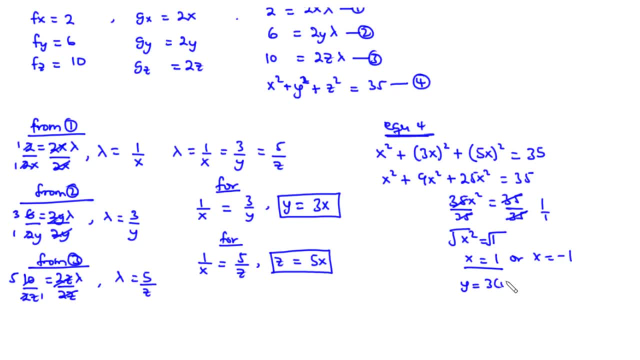 we are going to have y to be equal to 3 times 1, which is equal to 3, and then for x equals 1. also, we have z to be equal to 5 times 1, which is equal to 5. also, for x equals negative 1. we are going to have y to be 3 times negative 1, which is equal to. 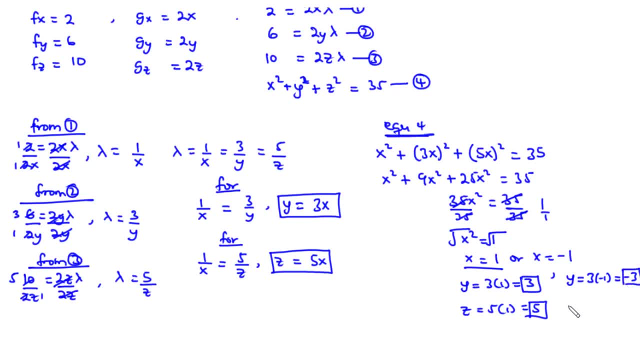 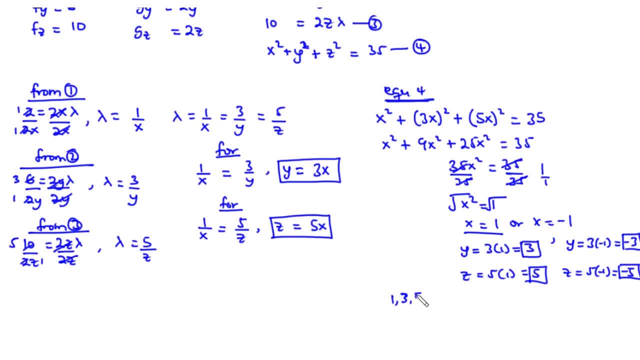 negative 3, and then also z equals 5 times negative 1, that is equal to negative 5. therefore, we obtain two points, which are 1, 3, 5, as well as negative 1, negative 3, negative 5. so these are the two points now we need. 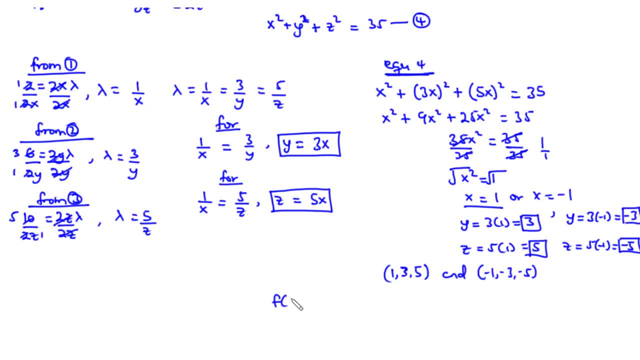 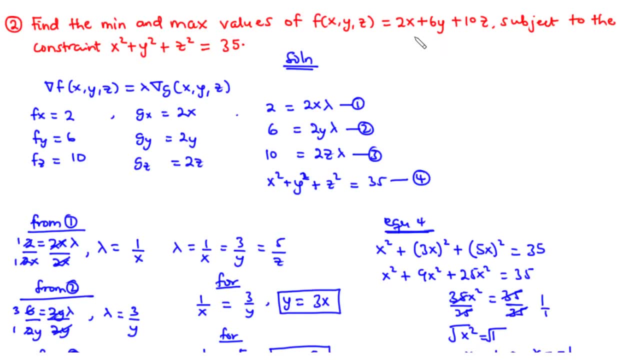 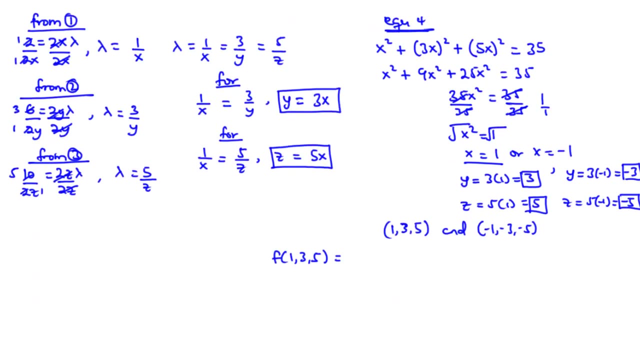 to find the value of the function at this point. so we have f of 1, 3, 5, that's equal to. we have the function to be 2x plus 6y plus 10z, 2x plus 6, y plus 10 z, 2. so 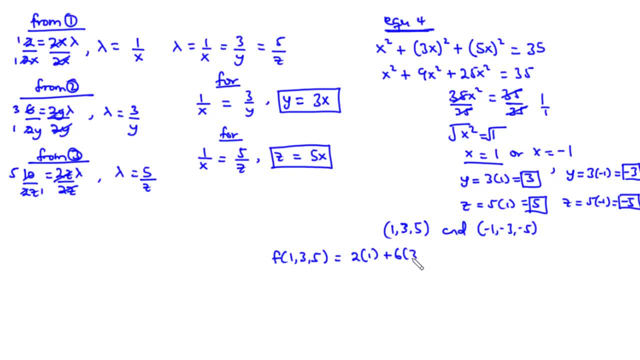 2 times x plus 6 times y plus 5 times z- sorry- plus 10 plus 10 times z, and that will be equal to. this is going to be 2 plus 18 plus 50, and that's equal to 2 plus 18. 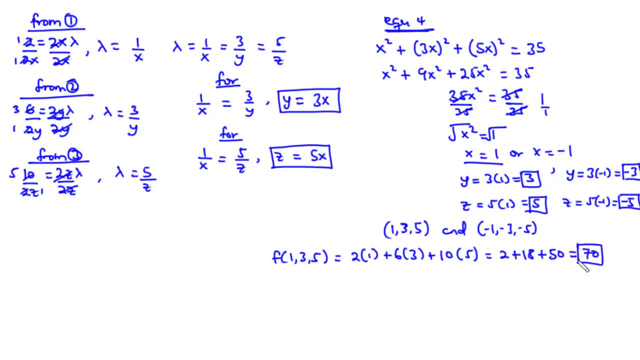 is 20 plus 50 is 70. so we have 7 cars in our system. we can figure out what we need to to be 70 and then f of negative 1, negative 3, negative 5, that will be 2 times negative 1 plus. 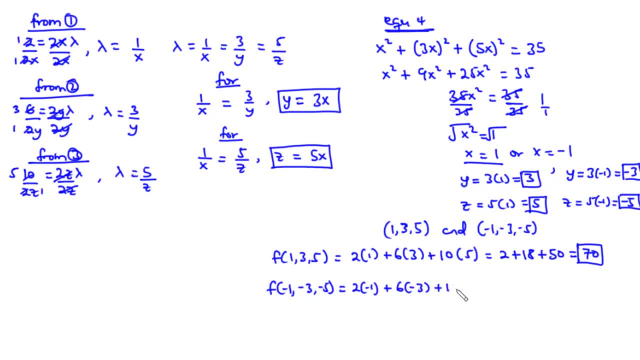 6 times negative 3 plus 10 times negative 5, that will be equal to negative 2 minus 18 minus 50 and that will be negative 70. So we have 70 to be the maximum value and occurs at the point 1,, 3,, 5. 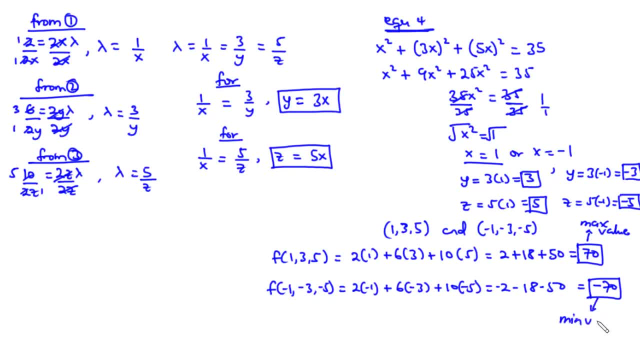 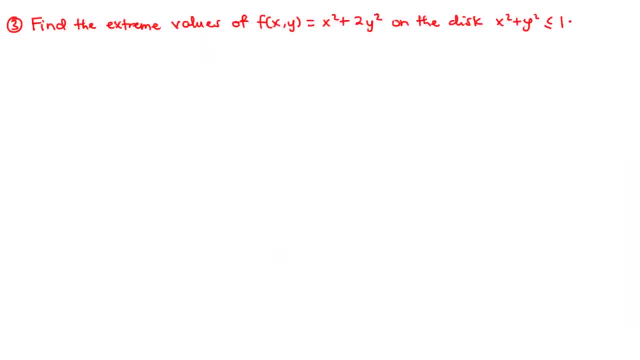 and then negative 70 to be the minimum value, and also occurs at the point negative 1, negative three, negative five. Now to example three. we are going to find the extreme values of the function f of xy on the disk x square plus y square, Esp. 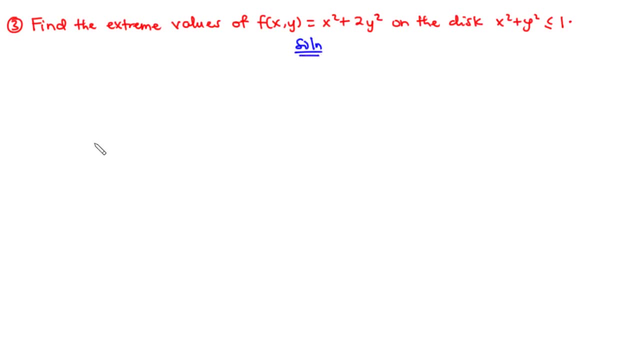 That we will be trying to solve in terms of building Simholder 2 andハ''f less than or equal to 1.. Now, in this example, the constraint is given by the inequality: x squared plus y squared is less than or equal to 1, which represents a closed and bounded region of a circle. 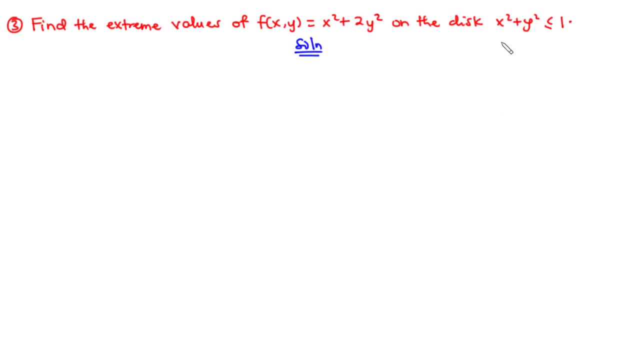 located at the origin. So for the equation of a circle located at the origin which has a radius r is given by: x squared plus y squared equals r squared. Now here we have the r squared part to be equal to 1 and that can be represented as 1 squared. Therefore we can have or we can say that: 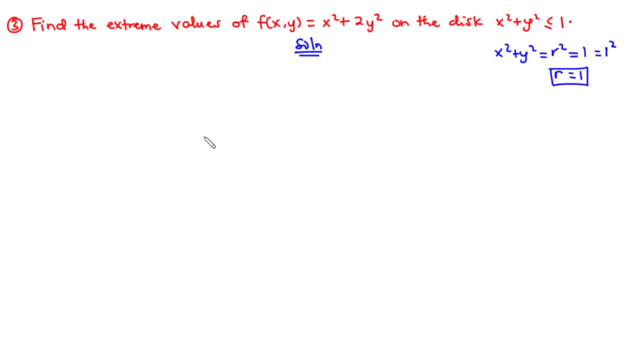 r is equal to 1.. We have r to be equal to 1.. Therefore, if we want to draw this circle, we have this to be the y-axis. the x-axis, radius is 1.. Therefore, we are going to have: 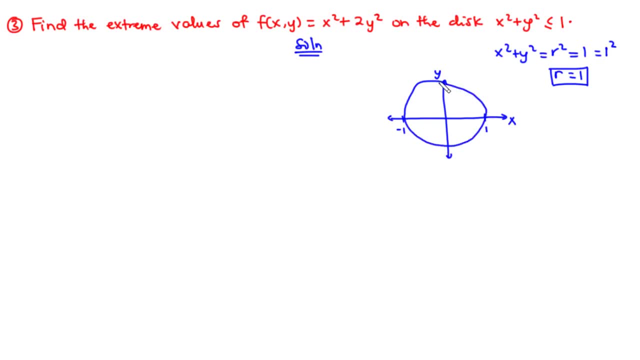 something like this, and then we have this to be the bounded region, including the boundary. Now notice that if we had x squared plus y squared equals 1, then we only focus on the boundary of this region, the boundary of the circle. However, 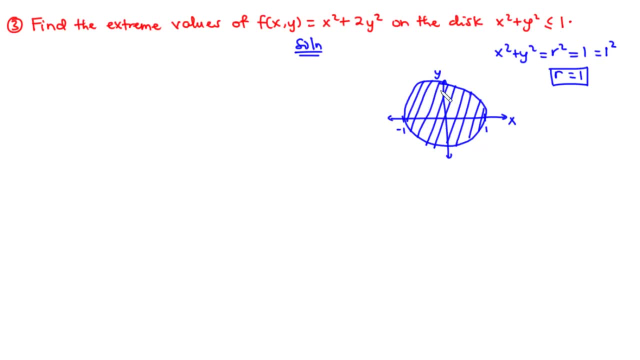 since we have, it's less than or equal to 1, it means that the interior of the region is also included. Now, in that case, it means that we need to find the critical point. So to find the critical point of this function, that is f, we first have f to be. 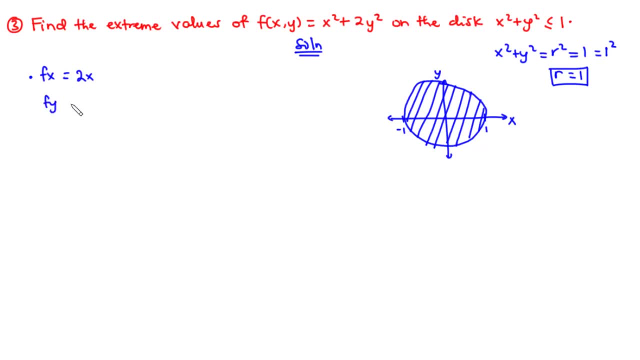 equal to 2x, and then we have fy also to be 4y. So after finding f, we are going to set each of them to 0. So we set this to 0, and thus we have x to be equal to 0, and then we also set: 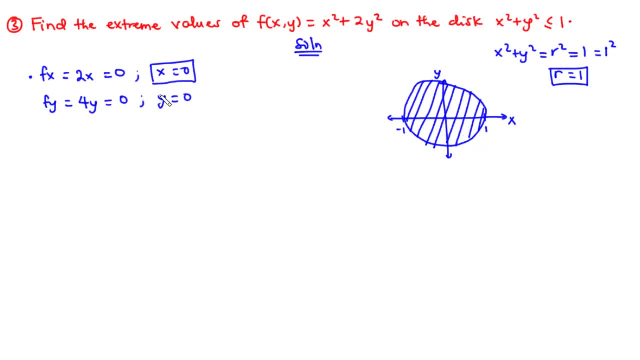 that to 0. and then we have y, also to be equal to 0.. Therefore we have the critical point 0,0.. And notice that this point is inside of this region. This is the origin, and hence we need to find the value of the function at this point. So we have f and that is equal to. 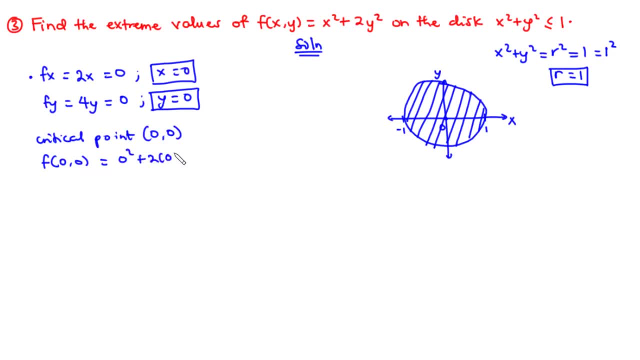 we are going to have 0 squared plus 2 times 0 squared, and that's equal to 0.. So the value of the function at the critical point is equal to 0.. Now, since we have f and then fy, we are going to find g and then gy. 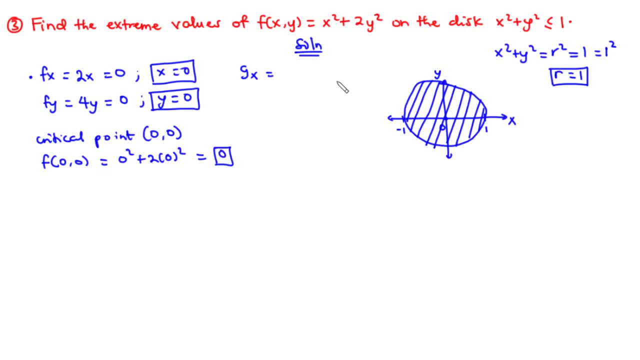 So we have g to be 2x and then we have g also to be 2y. Therefore, from the vector equation given by, the gradient of f equals lambda times the gradient of g, we are going to have f which is 2x. 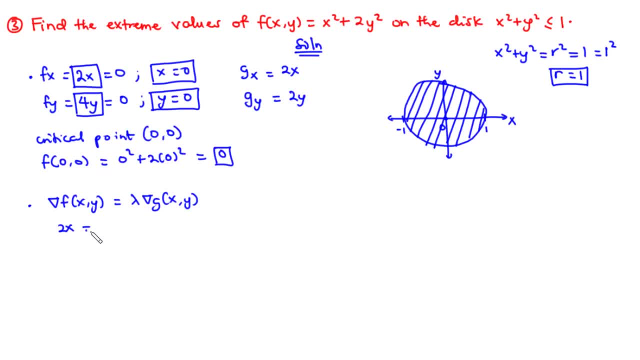 k times the gradient of f times 3y, which is 2y lambda. So we have 2x to be equal to 2x times lambda. let's call this equation 1.. We are also going to have 4y equals 2y lambda equation 2.. 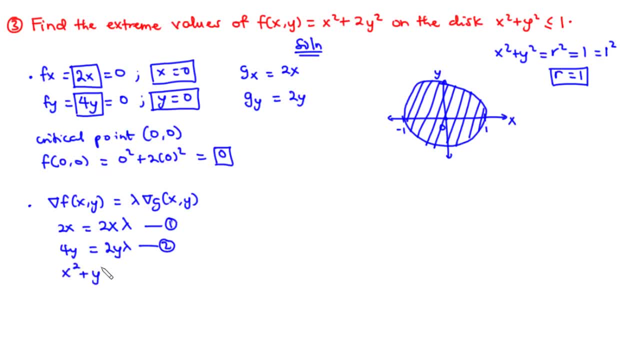 And then we have the constraints. Now, this time we are going to make this: x squared plus y squared equals 1. Instead of it's less than or equal to 1.. equation 3, so from: equation 1 and 2. let's modify equation 1 and 2, so from: 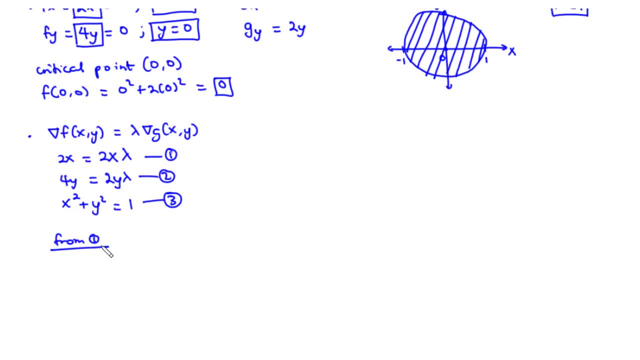 equation from equation 1. what we are going to do is we transpose 2x lambda to the left hand side. we have 2x minus 2x lambda equals 0. the greatest common factor is 2x. so inside of the bracket we have 1 minus lambda and that is equal to. 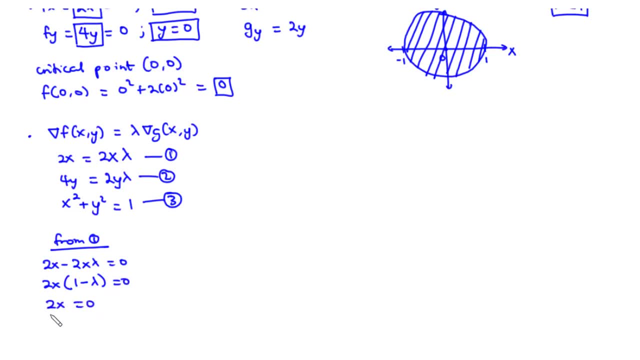 0. so here we have: 2x is equal to 0, we divide 3 by 2, and then we have X to be equal to 0. or we can also have 1 minus lambda equals 0, and then we find the value of lambda. but in this case we are not so much interested in the value of. 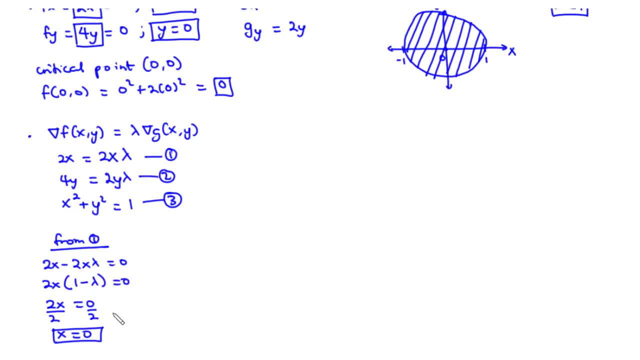 lambda. so we just ignore that. and then for X equals 0, we can put that into equation 3, so put: so we put X equals 0, put X equals 0 into equation 3, so when we do that, then we have 0 square plus y. 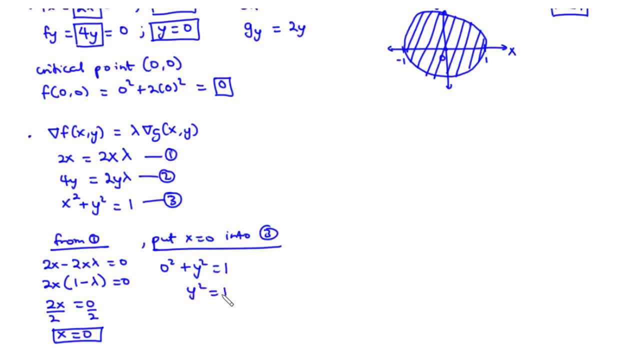 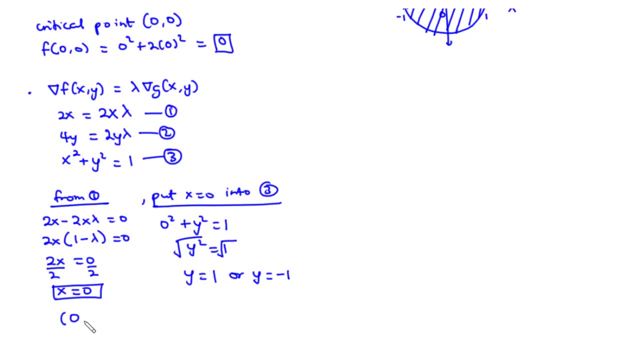 square is equal to 1. therefore we have y square equals 1. we take the square root of both sides and then we have y equals 1 or y equals negative 1. so at this point we have two points, which are the point 0- 1 and 0 negative 1. now so let's say this is a and then that is B. we are 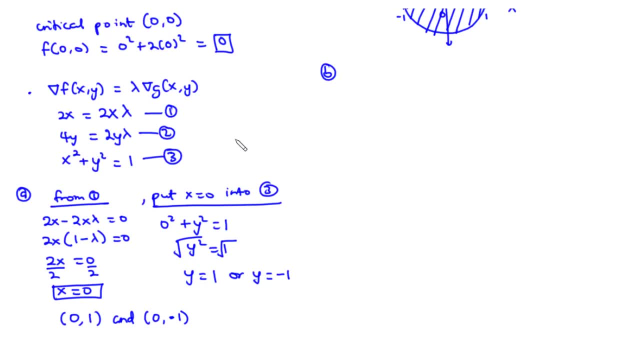 going to consider equation 2. now, from equation 2, that is from equation 2, we are going to have 4y minus 2y lambda equals 0. greatest common factor is 2y, so 2y out we have 2 minus lambda equals 0. we have 2y equal 0. we divide 3 by 2 and 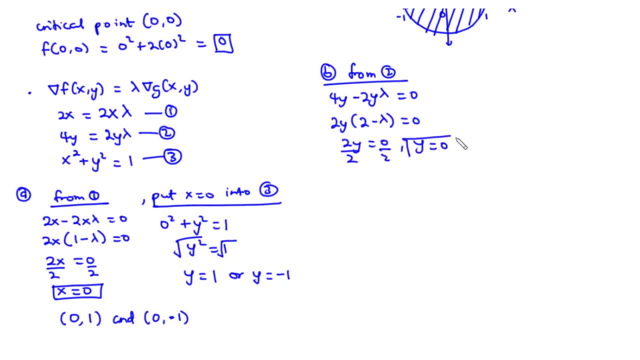 then we have y to be equal to 0. now we are going to put y equal 0 into equation 3 and then we are going to have x square plus 0. square is equal to 1, so is equal to 1.. Therefore we have x squared equals 1.. We take the square root of both sides and then 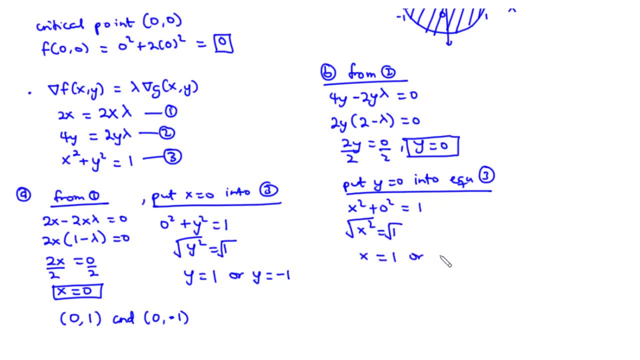 we have x to be equal to 1 or x to be equal to negative 1.. Therefore, we also have two extra points, which are 1, 0 and negative 1, 0.. So in all, we have four points. Now, the next thing we are: 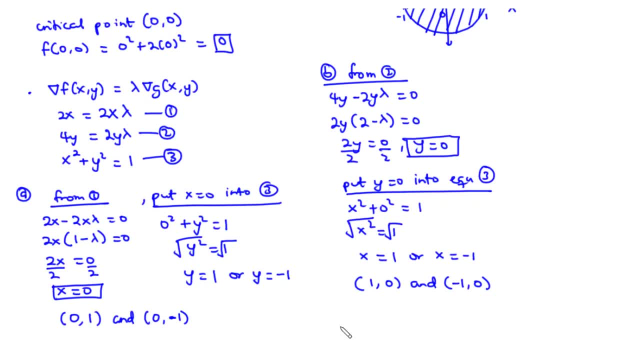 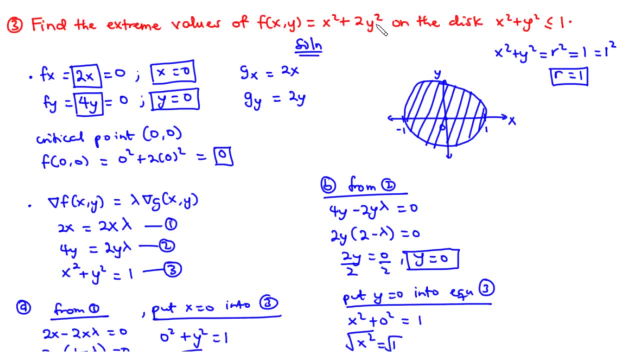 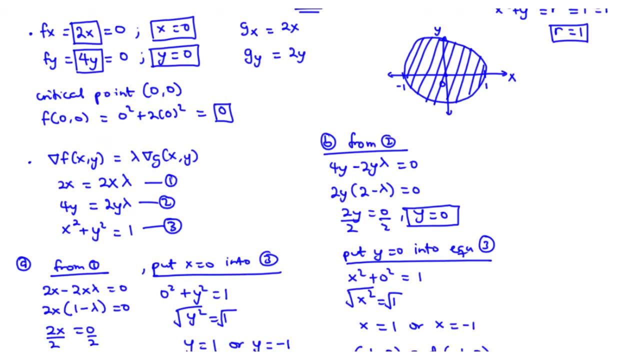 going to do is to find the value of the function at all these four points. Now, because we have f of x, y to be x squared plus 2, y squared, it means that for the negative values, the square takes care of them. So to find the values of the function at all these points, we have the function.